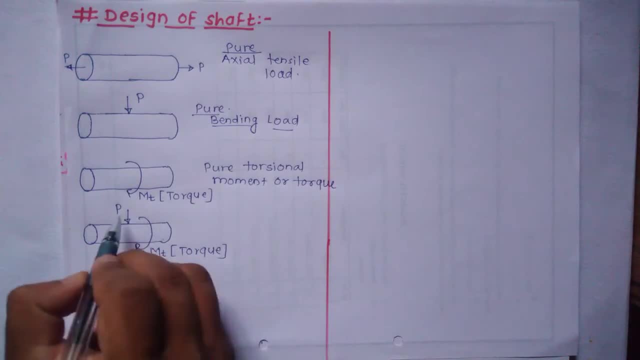 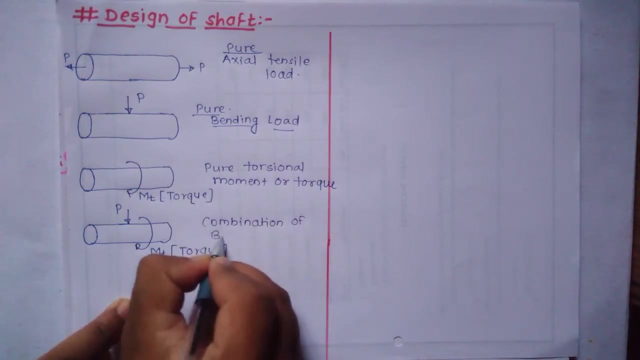 This is a somewhat complicated loading on the shaft where there is a bending load also and there is a twisting moment or torque also present in the shaft. So this is the combination of this type of loading conditions. The combination of this type of loading is the combination of bending load P, which cause the bending of this shaft. 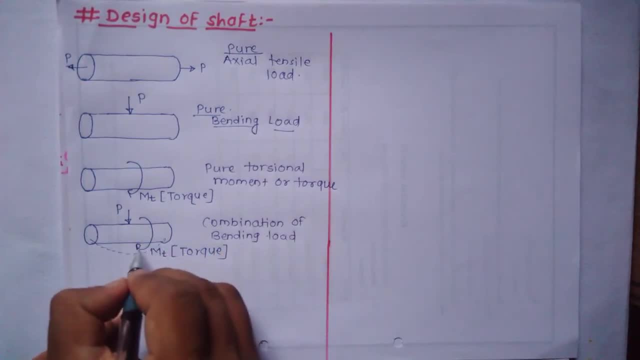 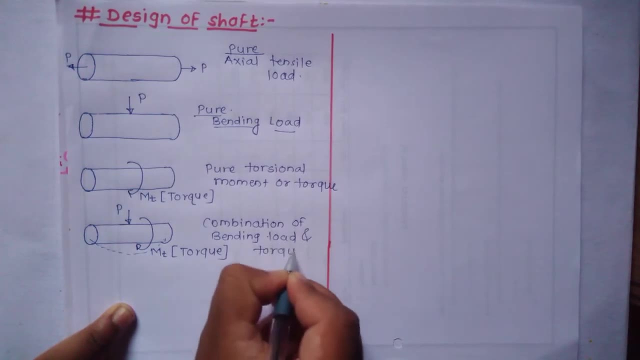 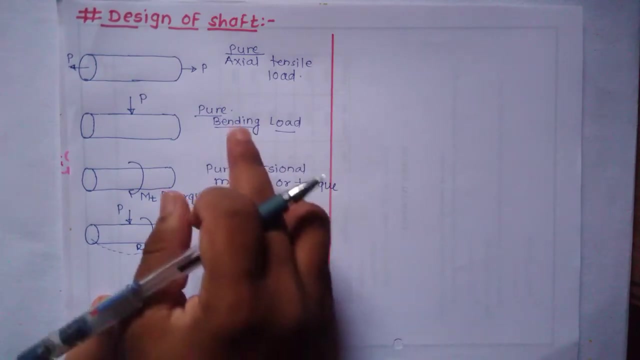 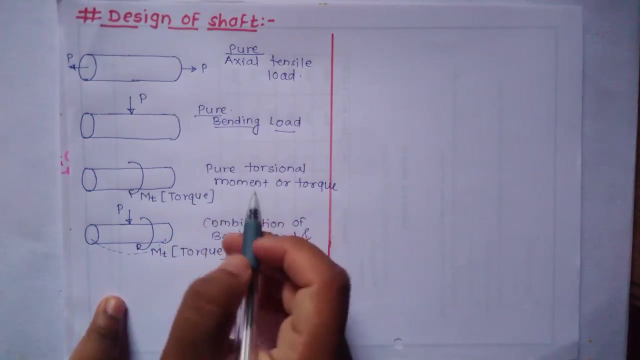 So combination of bending load and second is torsional moment or torque. So these are some of the examples of loading on the shaft. So we are going to consider each loading condition and we are going to find out what is the equation to find out the diameter of shaft in each loading condition. 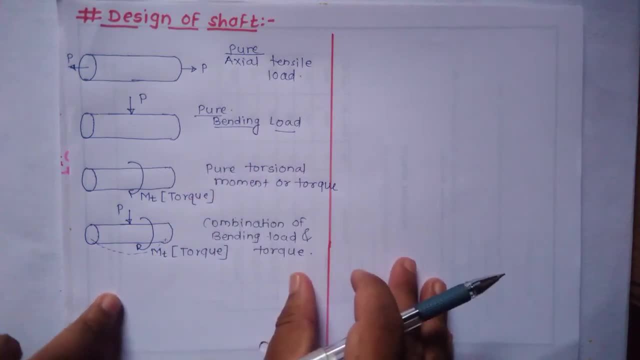 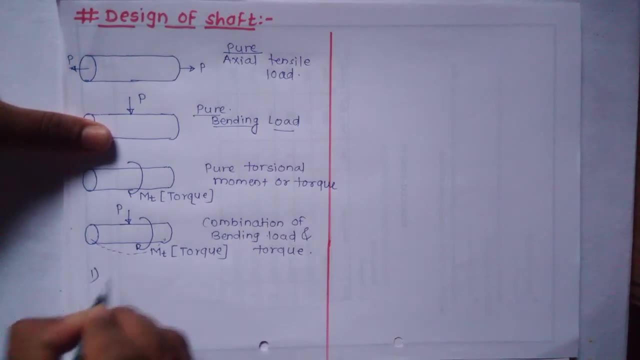 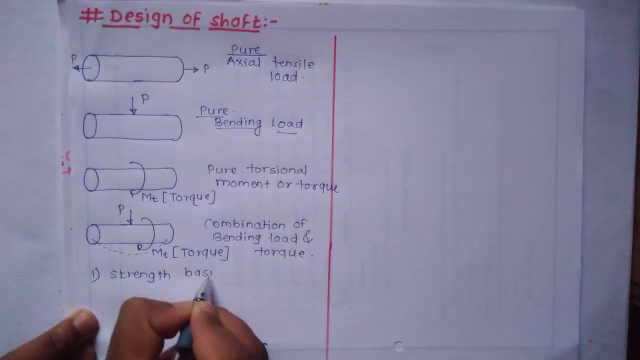 Now, basically, if you see, if you talk about the criteria to design the shaft, that is, to find out the diameter of shaft, there are two criteria. So first criteria is strength basis criteria. First criteria is strength basis criteria And second criteria is torsional rigidity criteria. 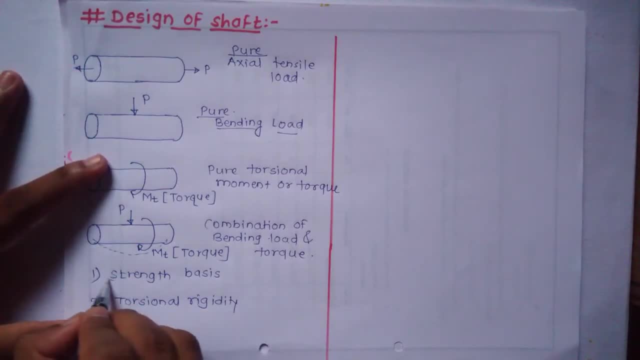 Now, this part is very interesting. Now, in the strength basis criteria, to find out the diameter of shaft, permissible stresses are used- Okay. So here permissible stresses are used To find out the diameter of shaft, Okay. And in torsional rigidity criteria, permissible angle of twist is used. 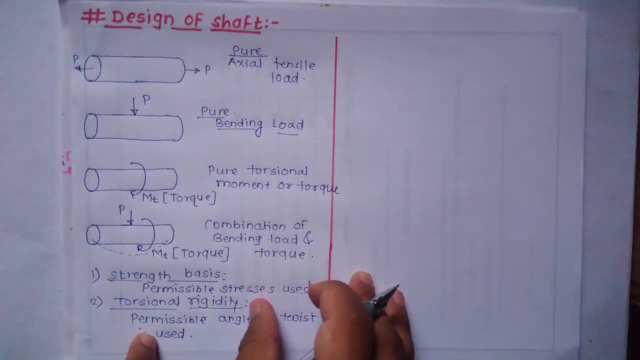 Now it is very important to identify the difference between these two criteria. Now the strength basis criteria. in this strength basis criteria, permissible stresses are used to find out the diameter of shaft. In most of the cases, permissible stresses are used to calculate the diameter of shaft, that is, to design the shaft. 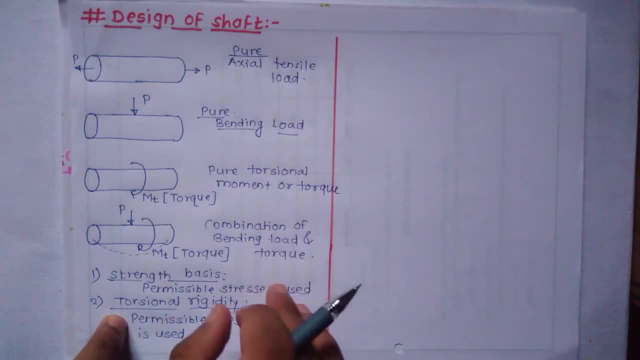 Now, as we know, that the shaft is subjected to different types of loading condition and because of that different stresses will induce in the shaft. So whenever the stresses are considered to design the shaft, it is known as strength basis criteria. Now the second criteria is torsional rigidity criteria. 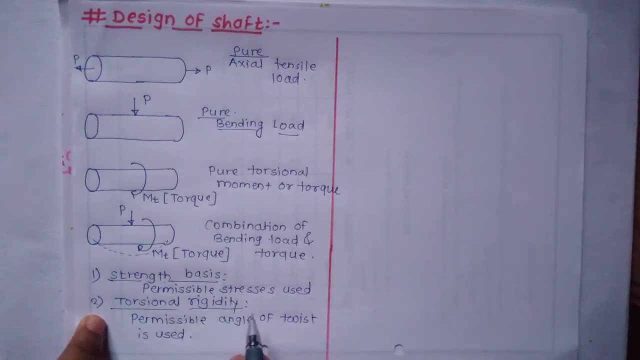 Now, in this torsional rigidity criteria, the permissible stresses are not considered to design the shaft, But the permissible angle of twist is used to design the shaft, that is, to find out the diameter of shaft. Now, in which cases this torsional rigidity criteria becomes important, 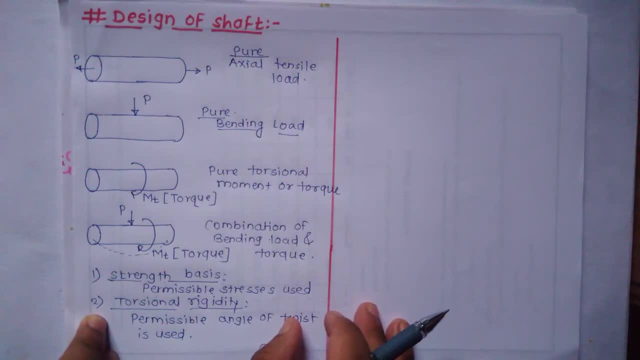 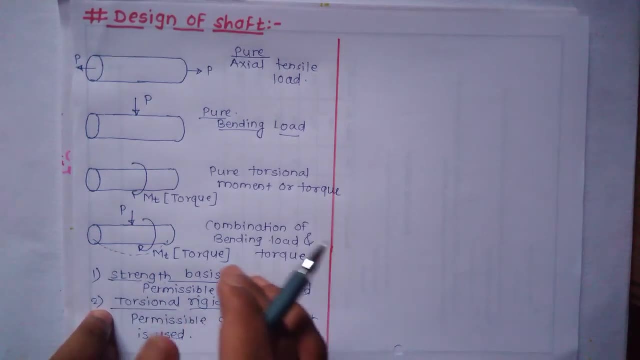 Now the certain applications where the length of shaft is very short. Okay, The length of shaft is very short. In such cases, the induced stress values are very low. Okay, The induced stress values are very less. Hence the possibility of failure of such short shaft is very less due to stress. 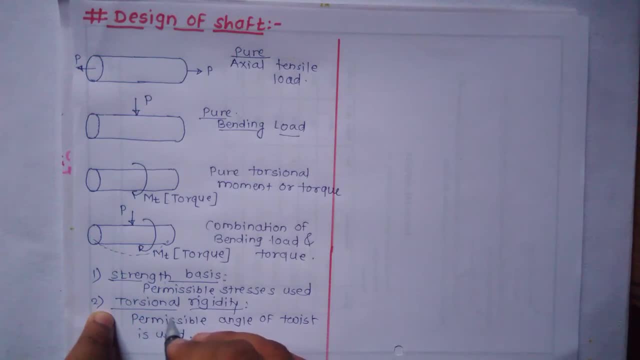 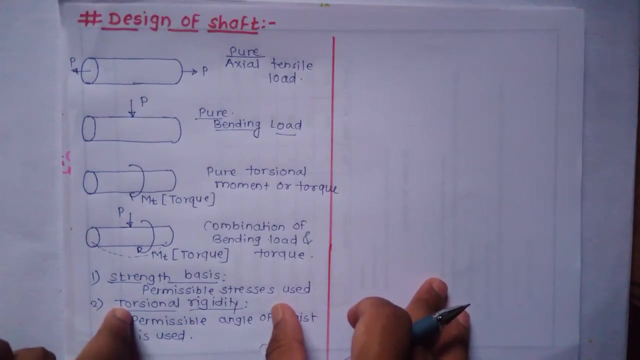 So in such cases the twisting becomes important criteria to design the shaft. So permissible angle of twist is considered in a shaft having shorter length Now in which applications the shorter shafts are used. So if you consider the examples of machine shaft, 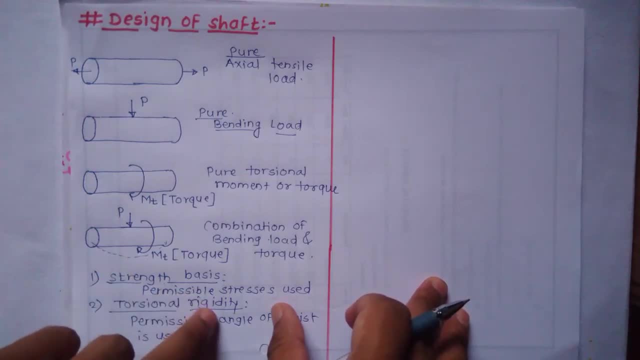 Okay, If you consider the example of lathe machine. So in the lathe machine spindle is used. It is a hollow shaft, So it is having shorter length. So in such spindle the stresses are very less because its length is very less. 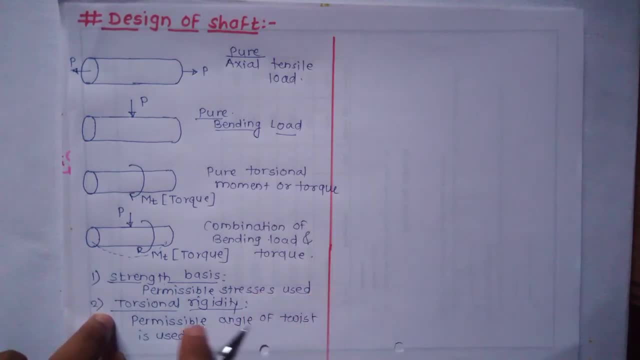 So what we can consider to design the shaft is permissible angle of twist, because there also the twisting occurs, And that is the criteria to design such a shorter shaft like a spindle in the lathe machine. Okay, So these are the two criteria. 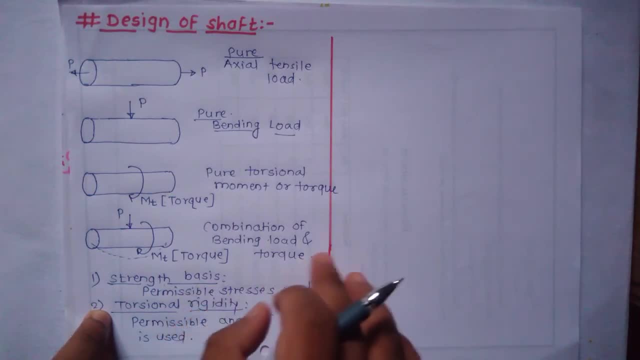 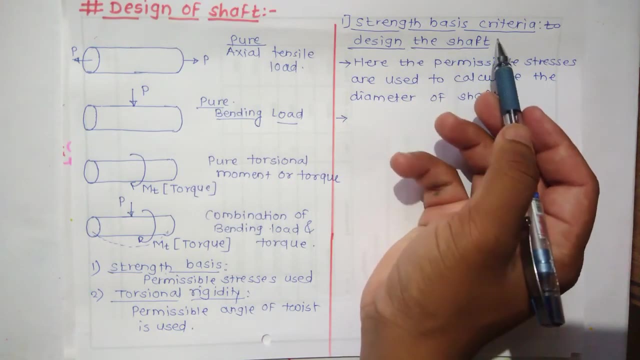 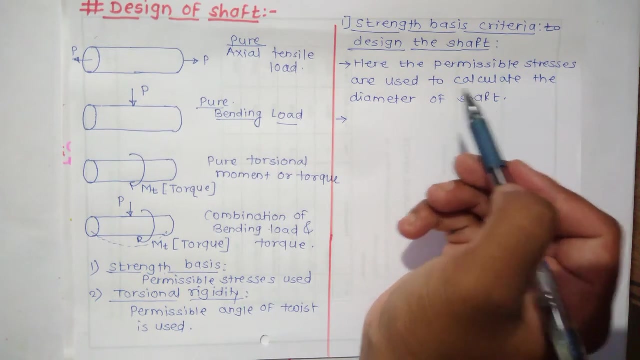 Now we will consider. Let us consider each criteria one by one with its equations. So, as we discussed in the strength basis criteria to design the shaft, the permissible stresses are used to calculate the diameter of shaft. Now there are different types of loading conditions like this: 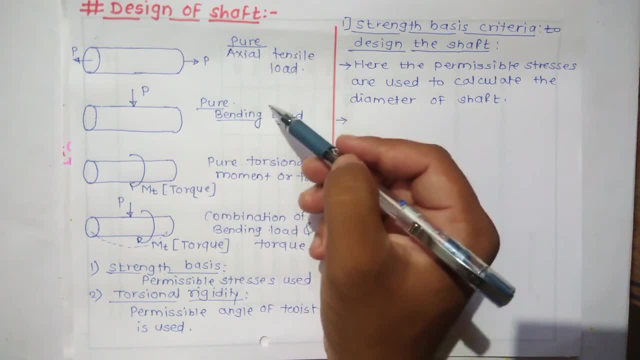 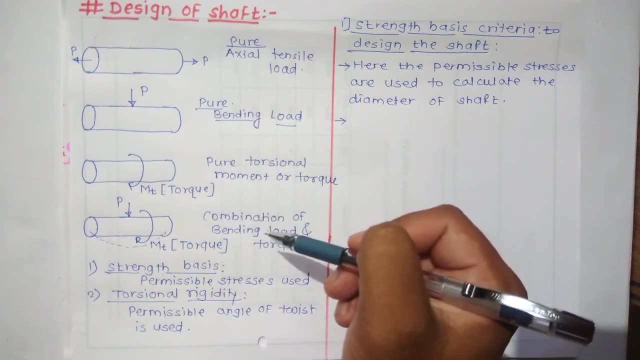 The shaft may be subjected to axial tensile load, The shaft may be subjected to bending load, The shaft may be subjected to only torsional moment or torque, Or shaft may be subjected to combination of loads. So now we have to consider each loading condition. 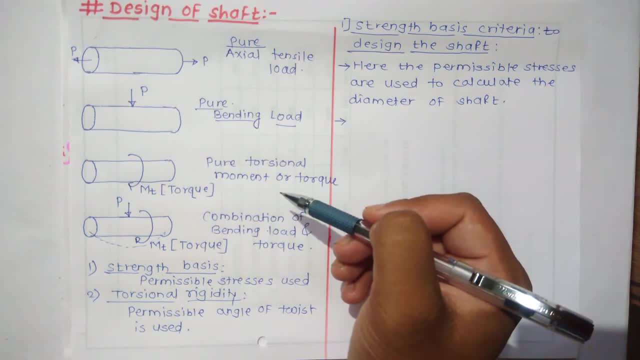 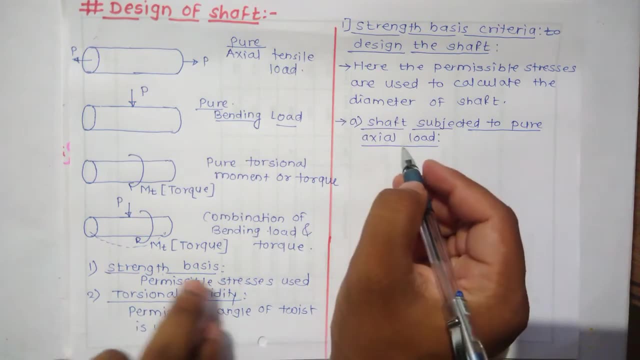 And we have to write the equation to find out the diameter of shaft. Now let us consider first the shaft subjected to pure axial load. Now let us consider this: is the shaft subjected to pure axial load If the diameter of shaft is D. 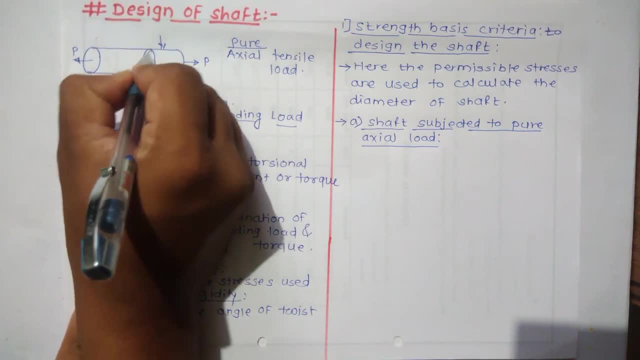 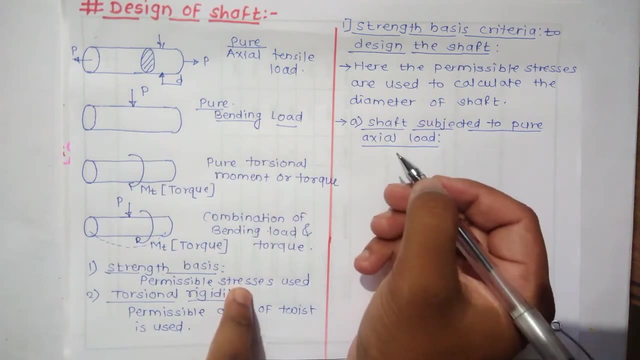 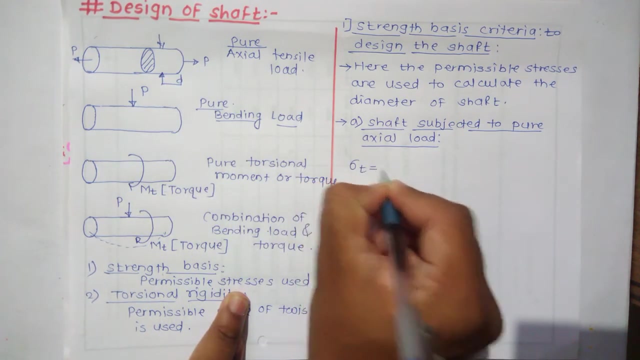 Okay, Then the cross section of this Shaft is circular, having diameter D. We can write the equation to find out the stress The tensile stress will induce because of this axial tensile load. So we can write the equation for tensile stress, which is given by sigma T is equal to P upon pi by 4 D square. 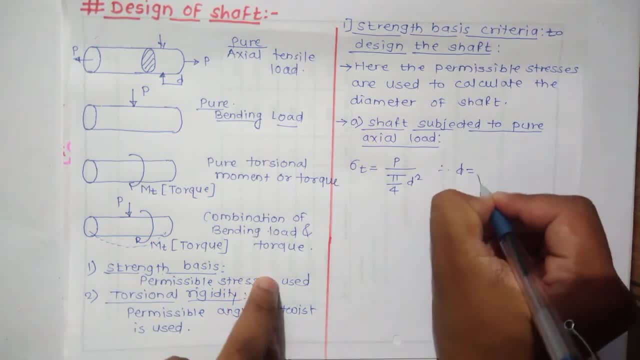 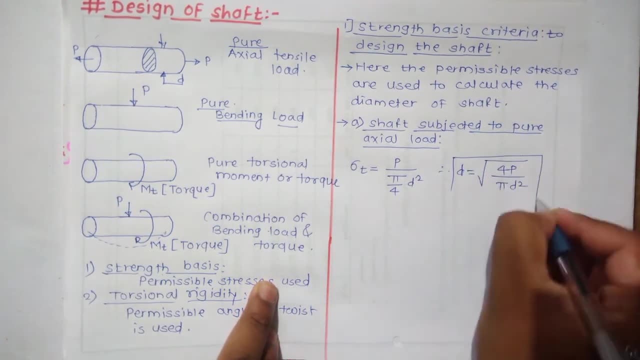 Okay, So from this equation we can easily find out: the diameter of shaft. D is equal to under root 4P upon pi D square. Okay, D is equal to under root 4P upon pi D square. Now in this equation, if we put the value of external load, P, 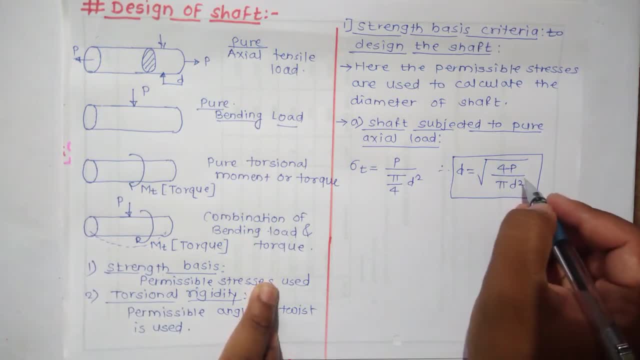 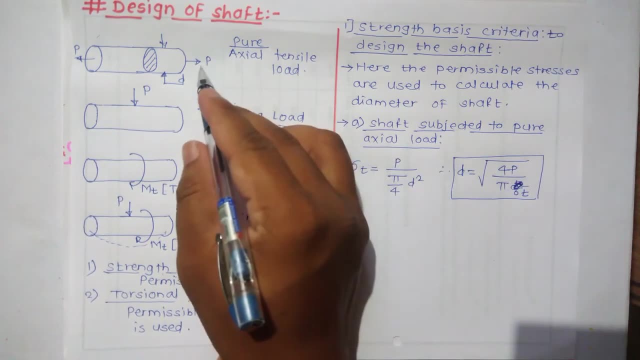 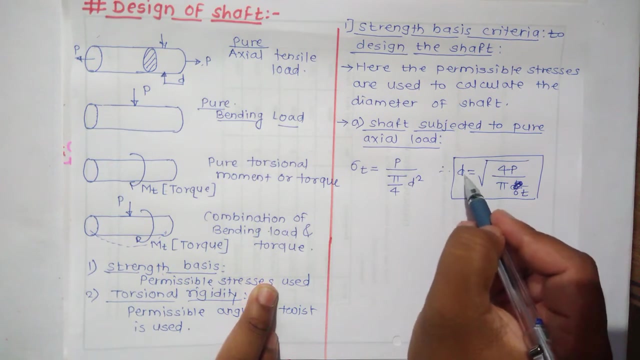 If we put the value of- Sorry, here, sigma T must be there. So if we put the value of P- external load, External tensile load- If we put the value of permissible tensile stress here, We can easily calculate this diameter of shaft. 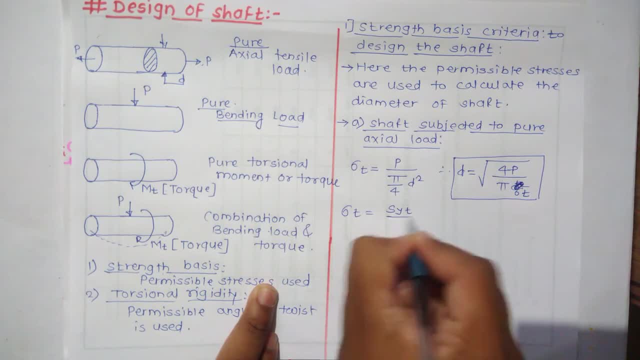 And this permissible tensile stress can be calculated from the equation SYT upon FS, Where SYT is the yield strength in Newton per mm square And FS is the factor of safety. So with this equation we can find out the diameter of shaft subjected to pure axial load. 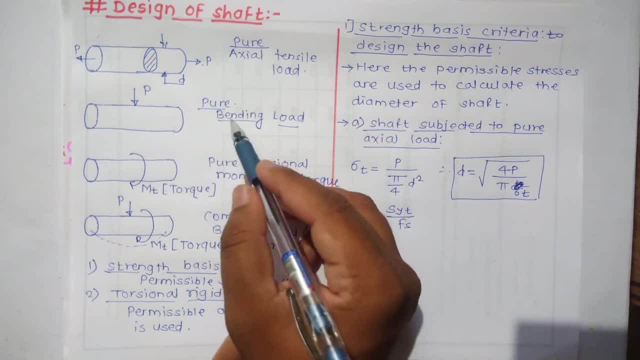 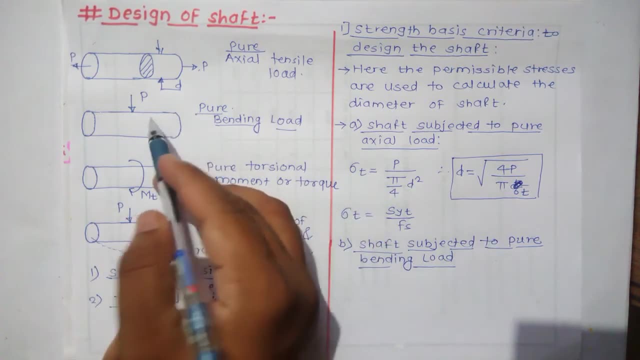 Now let us consider the second case, When the shaft is subjected to pure bending load. Now let us consider the shaft subjected to pure bending load, And this is the diagram for shaft subjected to pure bending load. Now, if the D is the diameter of shaft, 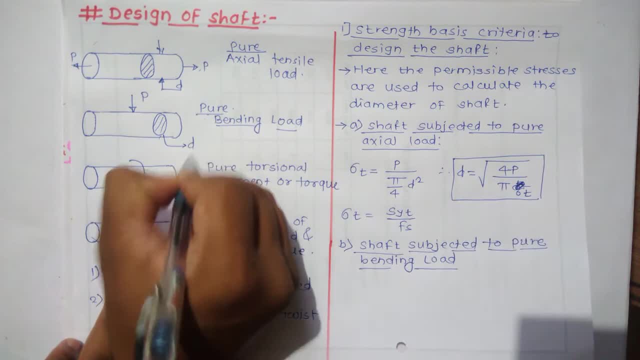 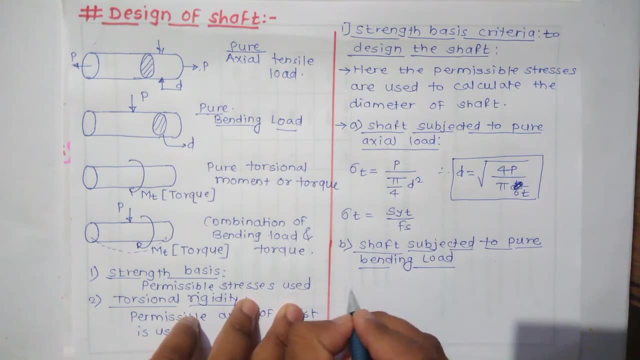 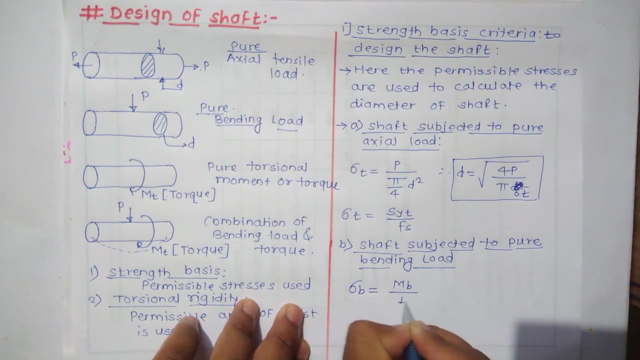 Okay, If D is the diameter of shaft, Then we can write the bending stress equation for this case, Where the shaft is subjected to only bending load, So bending stress is given by sigma B is equal to MB upon I into Y, So where this MB is nothing but the maximum bending moment. 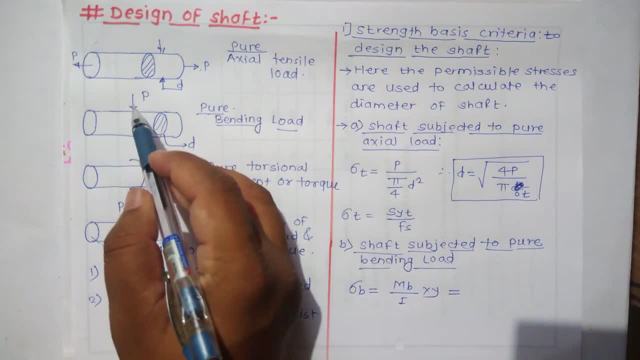 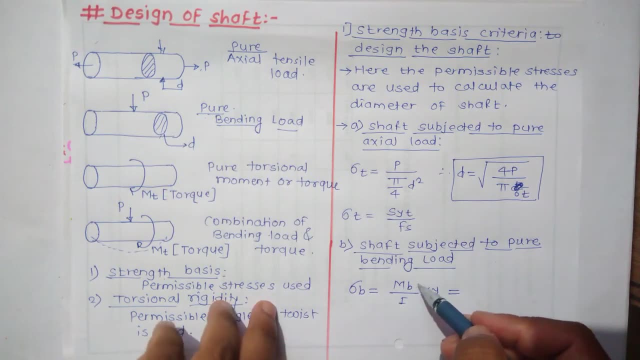 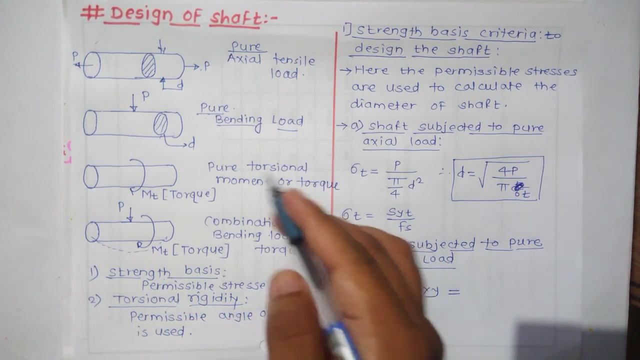 Now it depends on the external loading. Okay, So where is the maximum bending Moment? So that bending moment can be calculated on by considering the loading on the shaft. This, I, is nothing but the moment of inertia. So if the shaft is solid, 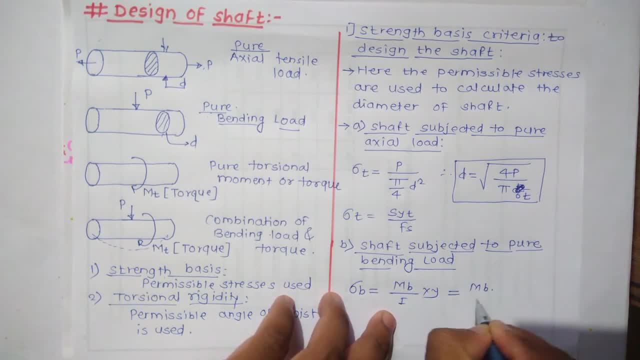 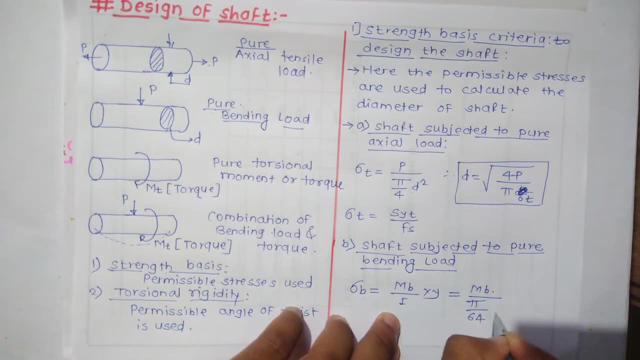 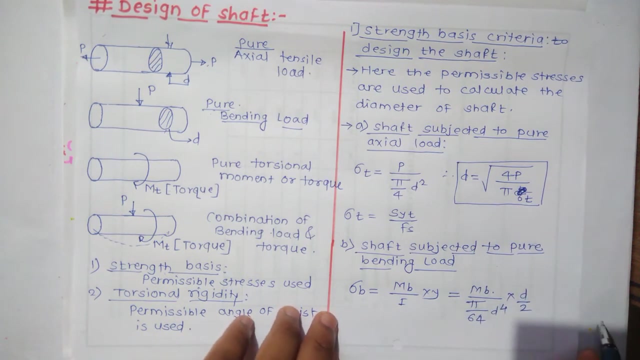 We can write the moment of inertia as pi, by 64, D raised to 4.. And we can write Y as D upon 2.. Okay, So in this equation, If we put the value of permissible bending stress, Which can be taken as equal to permissible tensile stress, 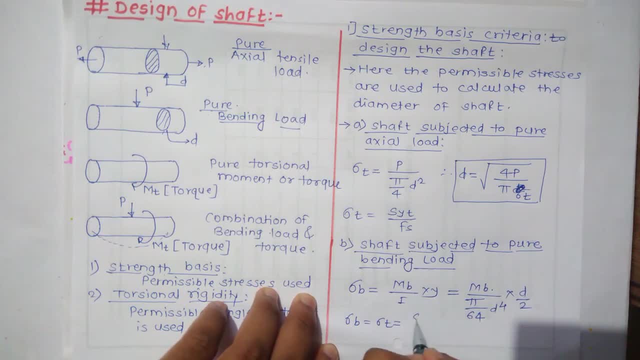 And we know that permissible tensile stress can be calculated as SYD upon FS. Okay, So if we put in this equation The value of permissible bending stress equal to permissible tensile stress, If we put the value of bending moment MB, 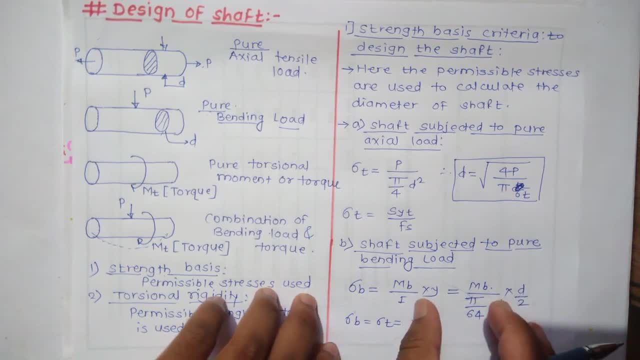 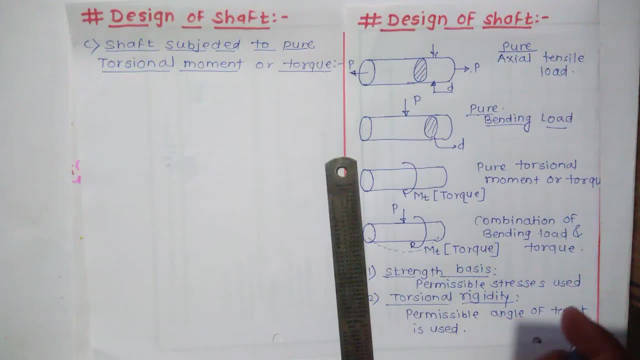 We can easily calculate the diameter of shaft D. Okay, So in this way we can find out the diameter of shaft Which is subjected to only bending load. Now let us consider the third loading condition, That is, pure torsional moment or torque. 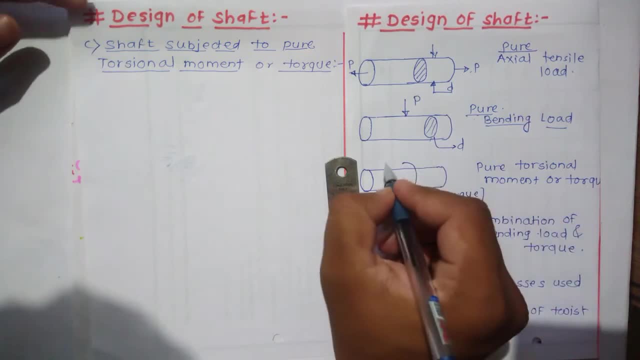 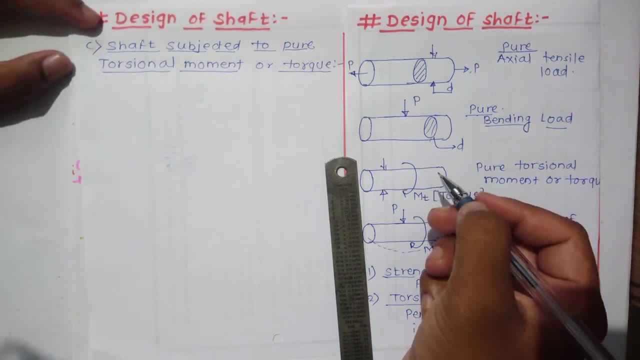 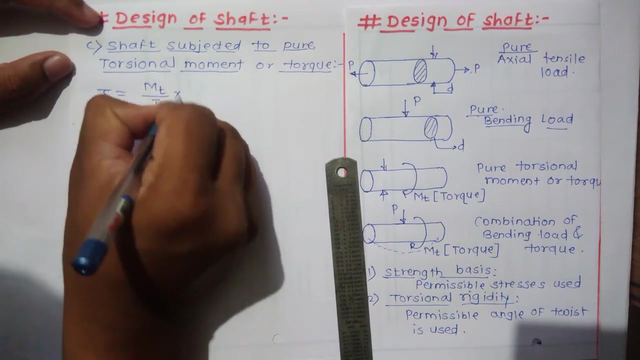 Now, when the shaft is subjected to pure torsional moment or torque having diameter D, The type of stress induced in the shaft is torsional shear stress, Which is denoted by tau. So torsional shear stress in this shaft can be given by equation MT upon J into R. 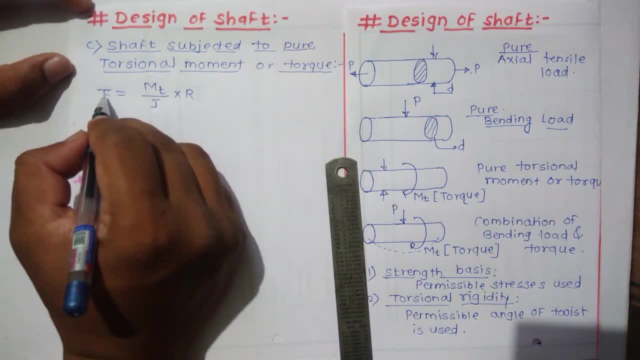 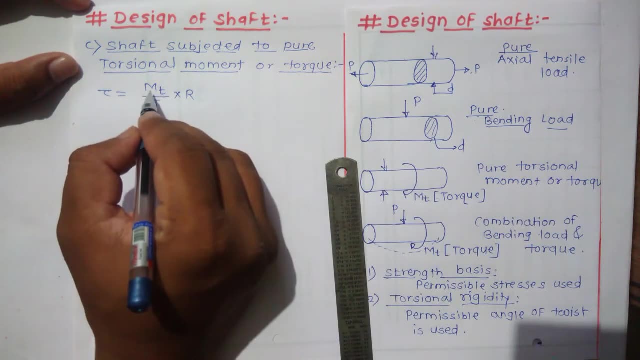 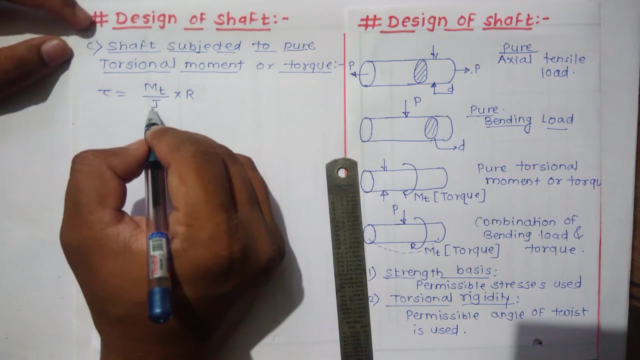 Where this tau is the induced shear stress, torsional shear stress in the shaft, Which is subjected to only torque or torsional moment. MT is the external torque or torsional moment in newton. mm. J is the polar moment of inertia, in mm. raise to 4.. 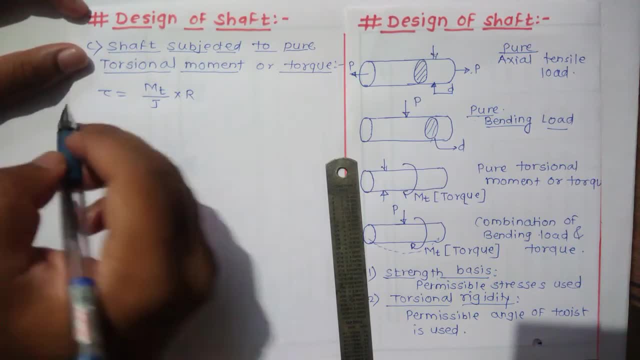 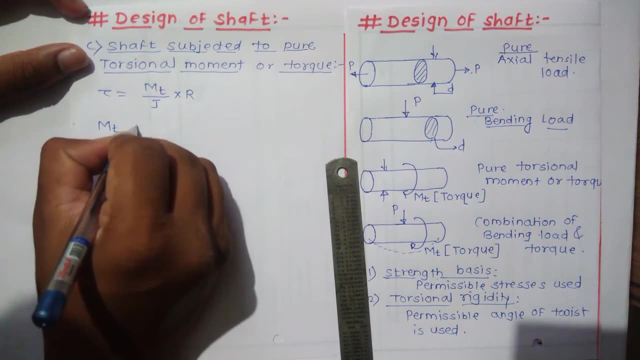 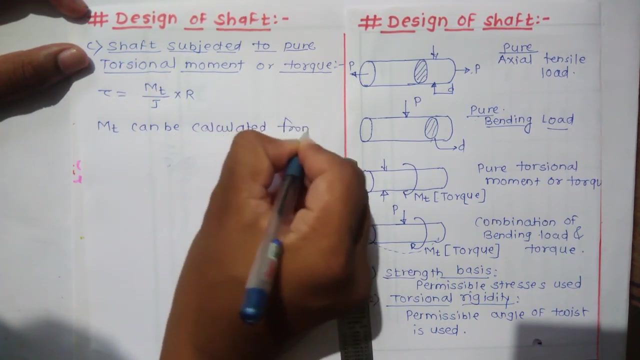 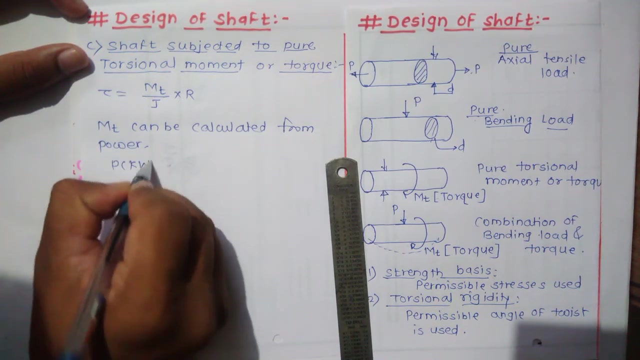 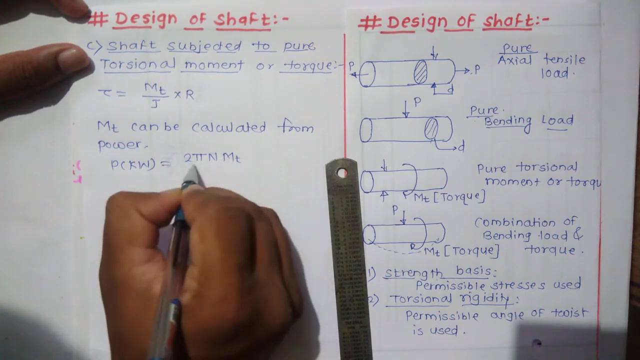 And R is the distance from neutral axis. So we can write here This: MT can be calculated from power. MT can be calculated from power. So if the power is known We can calculate this. tau, That is, P in kilowatt is equal to 2 pi N MT upon 16 to 10 raise to 6.. 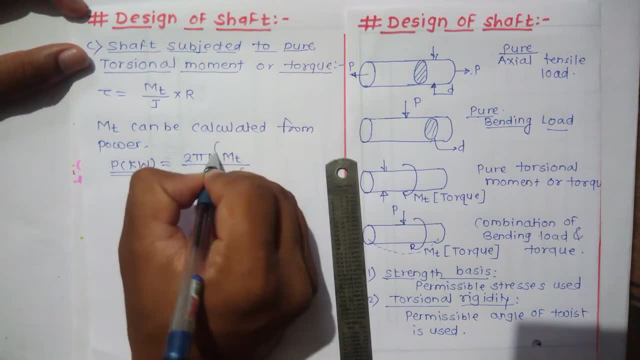 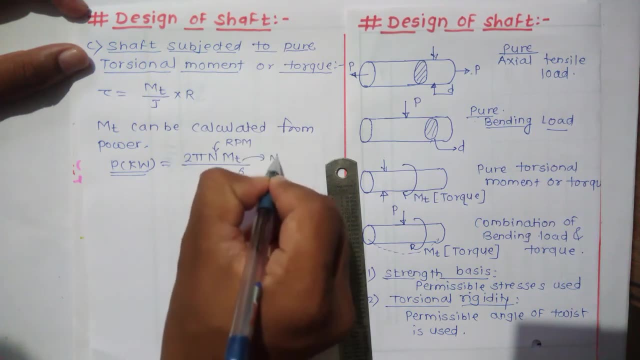 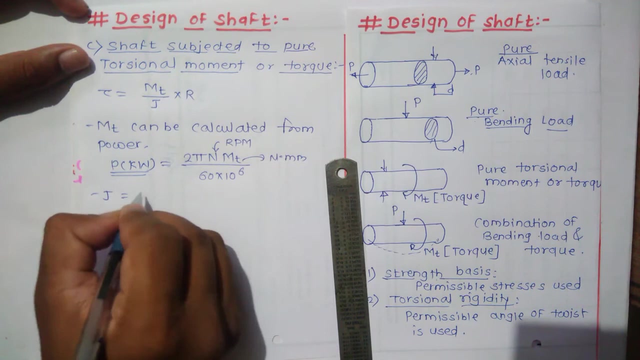 So if power is given in kilowatt, If RPM is given, Then we can easily calculate this torque in newton mm. Next is this J. So J we can express in terms of diameter, D. So pi by 32, D raise to 4.. 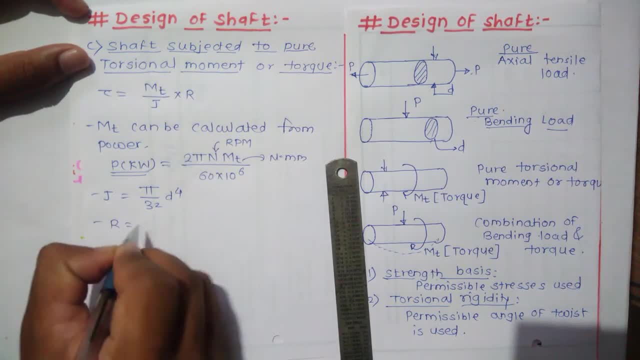 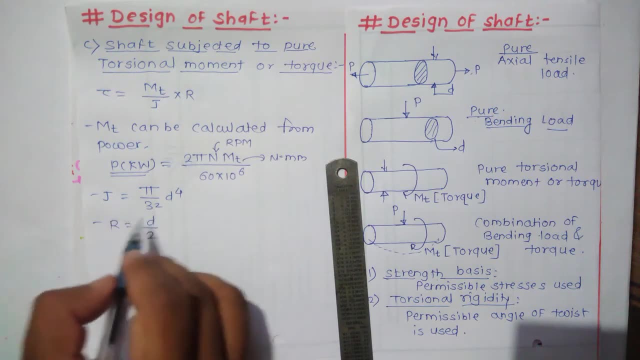 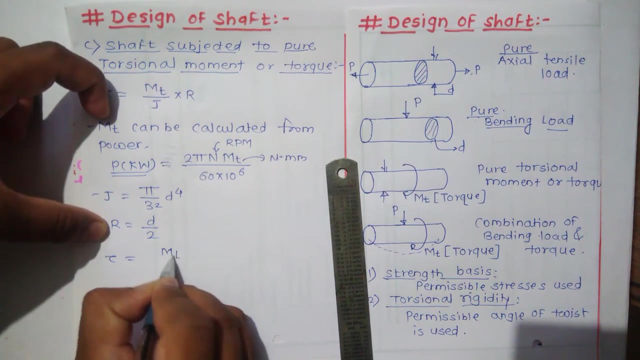 And this R can be expressed again in terms of D. It is D upon 2.. So it is a radius. Now if you put this value of J R In this equation, We get this equation like this: So tau is equal to MT upon pi by 32. D raise to 4 into radius D upon 2.. 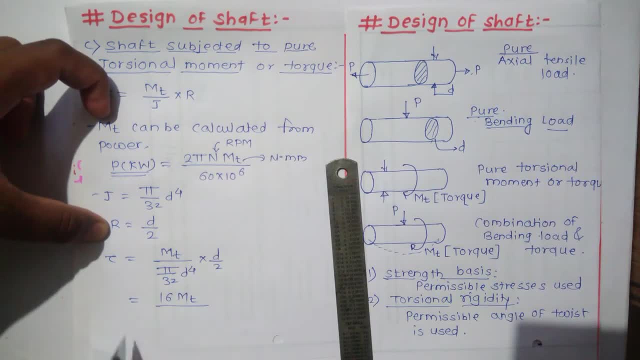 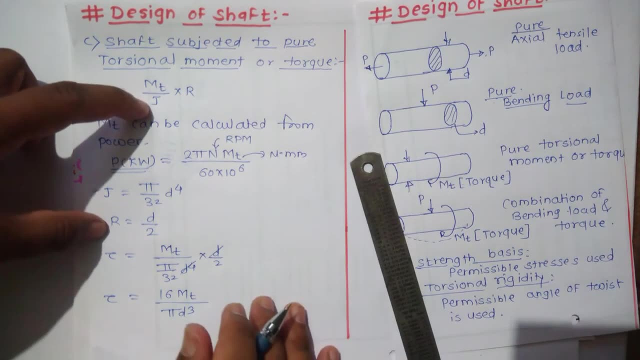 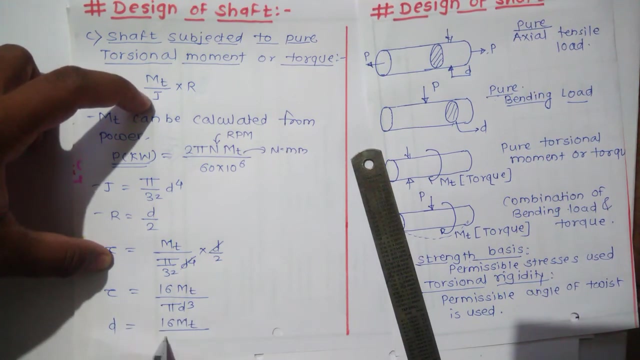 So we get this equation as 16 MT upon pi D cube. So from this equation We can write the equation to calculate diameter. So D is equal to 16 MT upon pi D cube. So from this equation We can write the equation as 16 MT upon pi into tau. 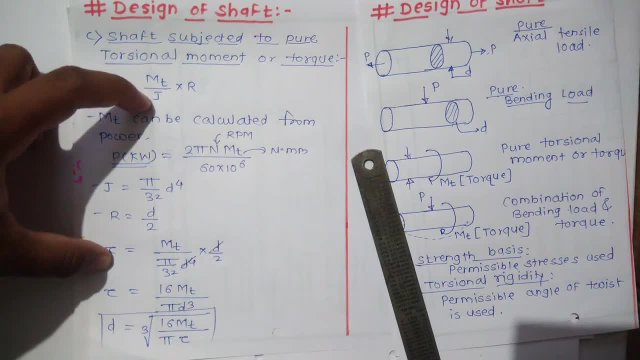 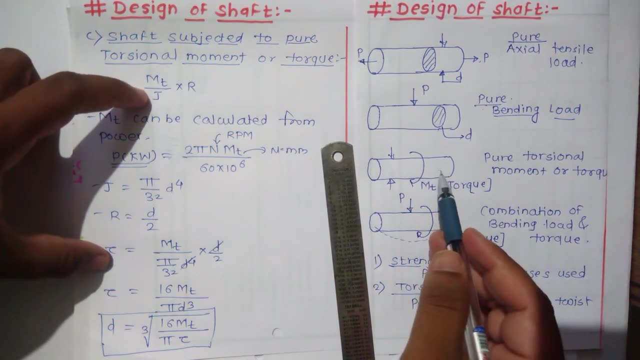 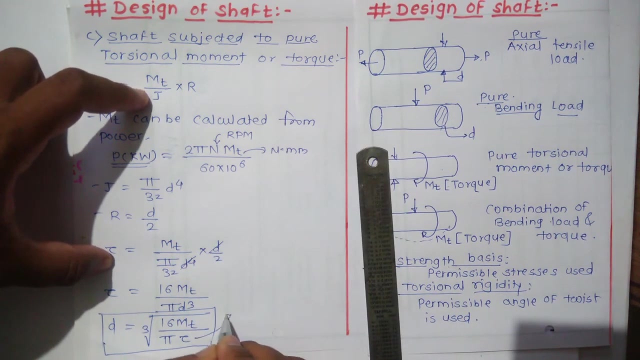 And this is in cube root. So this is the equation to calculate the diameter of shaft, Where the shaft is subjected to only torsional moment or torque, So where this tau is nothing but the permissible shear stress. So if we put the value of permissible shear stress here, 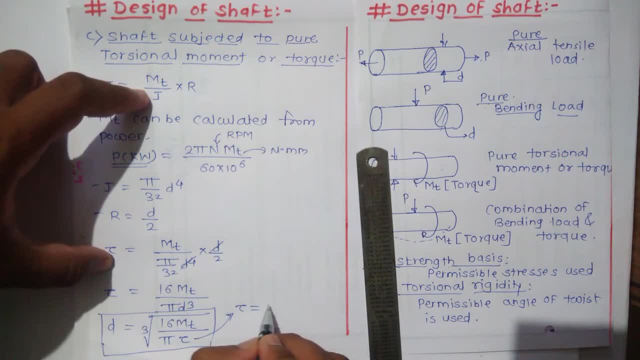 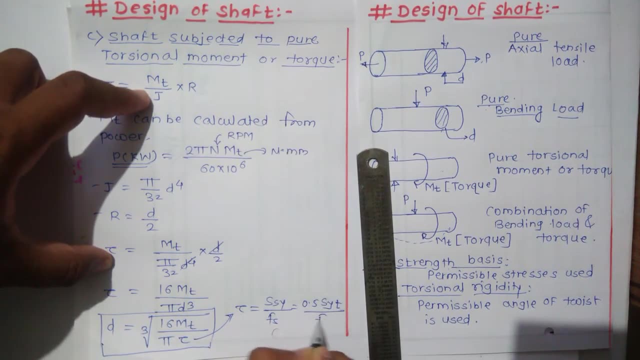 We can calculate this diameter So tau, that is permissible shear stress, can be calculated by using equation SSY upon Fs, where ssy can be calculated as 0.5 syt upon fs, where syt is yield strength in tension and fs is 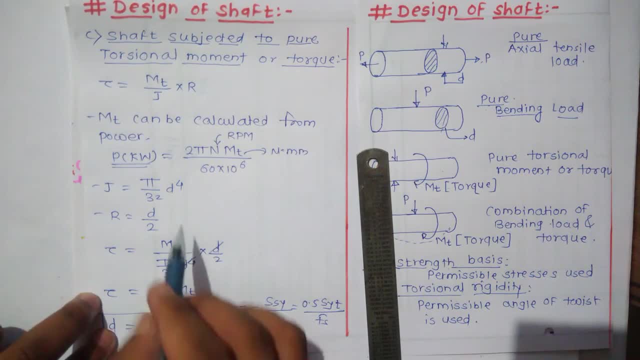 factor of safety and mt. already i have explained how to find out this empty. so p in kilowatt is equal to 2 pi and mt upon 16 to 10 raise to 6, where power it is in kilowatt and it is rpm that. 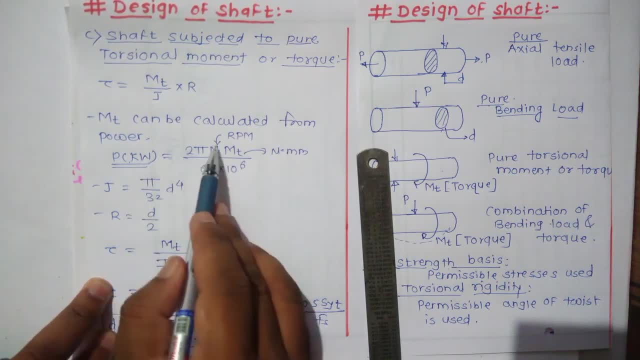 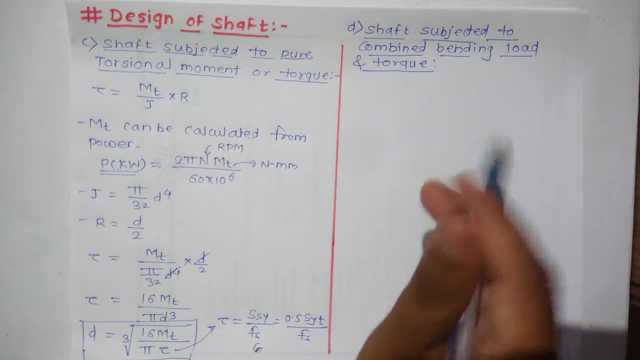 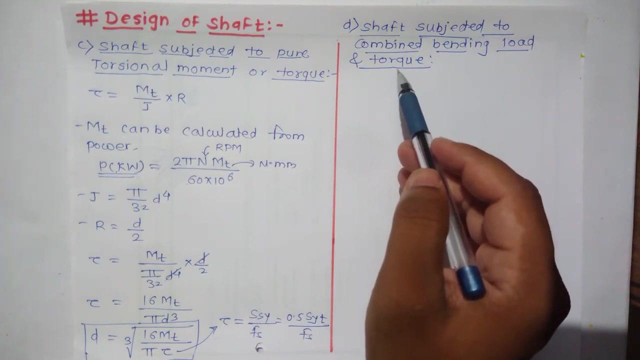 is a revolution per minute of shaft, and if power is known, rpm is known, we can calculate torque in newton mm. now, the last case in this strength basis criteria is the shaft subjected to combine bending load and torque. this torque is also known as torsional moment. okay now, as shown in this, 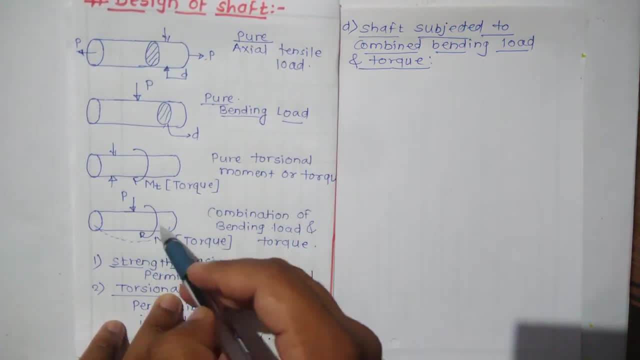 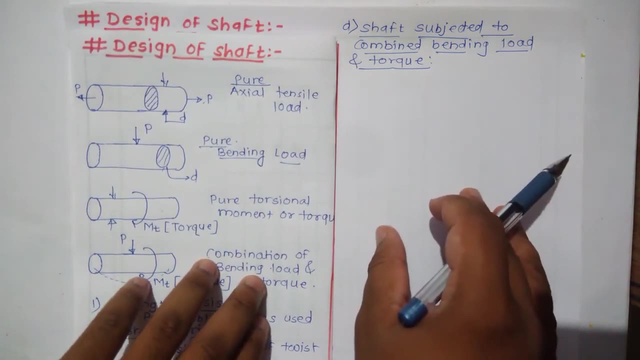 figure if the shaft is subjected to bending load p and torsional moment or torque mt, we have to use a different approach, okay, so here this type of analysis is slightly complicated, because here we have to consider the material of torque, which is not the torque which is being applied in the 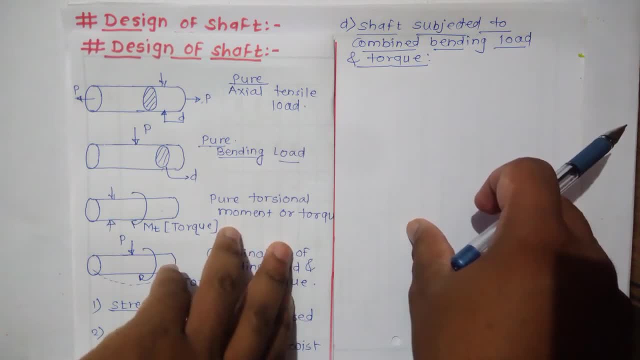 shaft. if the material of shaft is brittle, we have to use the maximum principle stress theory to design the shaft, and if the material of the shaft is a ductile, we have to use maximum shear stress theory. so first of all, consider the material of shaft is a brittle and let us write the equation. 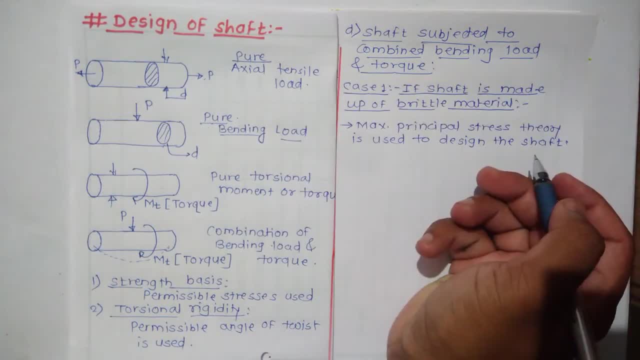 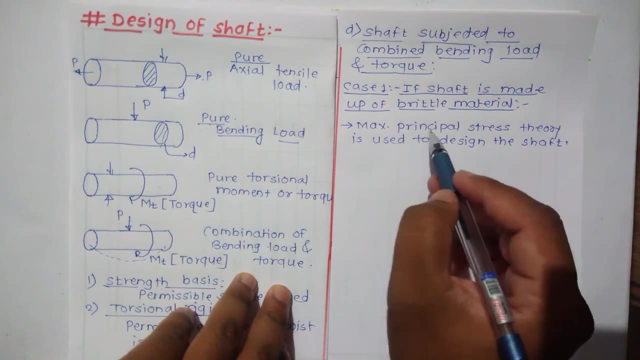 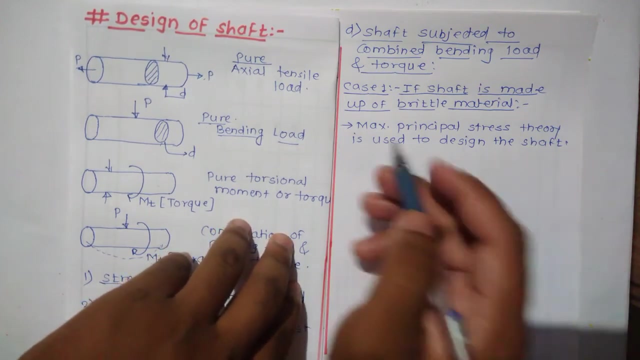 for maximum principal stress. now consider the case number one. if the shaft is made of brittle material? now, the shaft is made of a brittle material, we have to use the maximum principle stress theory to design the shaft, that is, to find out the diameter of shaft now, according to maximum principle stress theory, the maximum 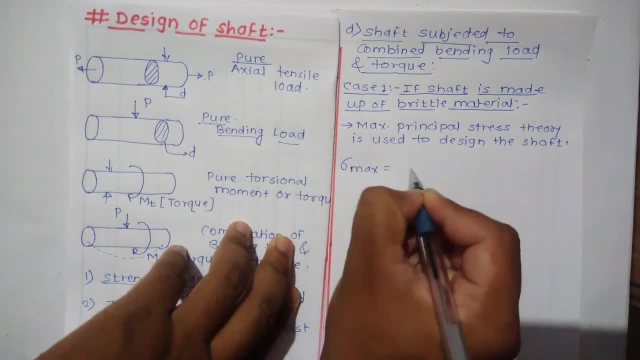 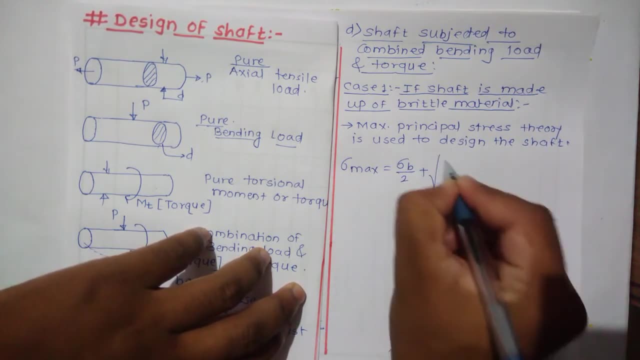 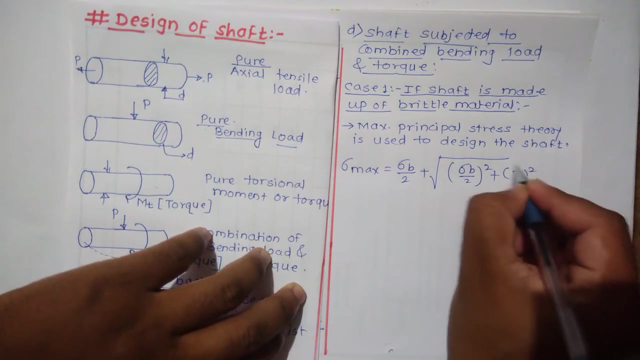 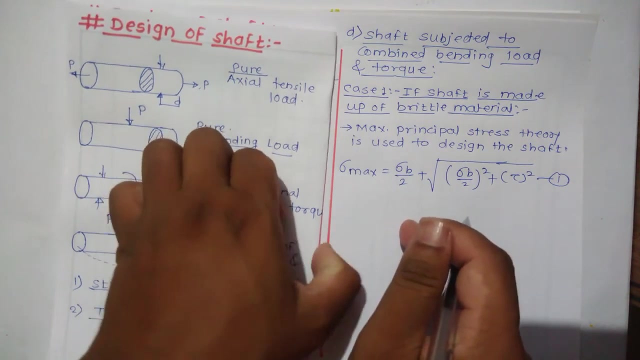 principle stress is given by equation: sigma max is equal to sigma b upon 2 plus, under root, sigma b upon 2 bracket square plus tau square. this is equation number one. so now already we have derived the equation of bending stress in the in the previous steps. so bending stress was: 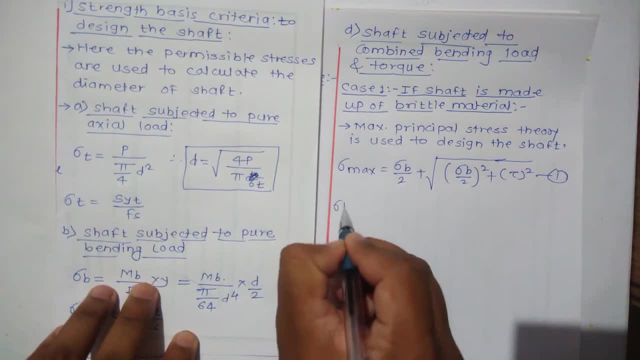 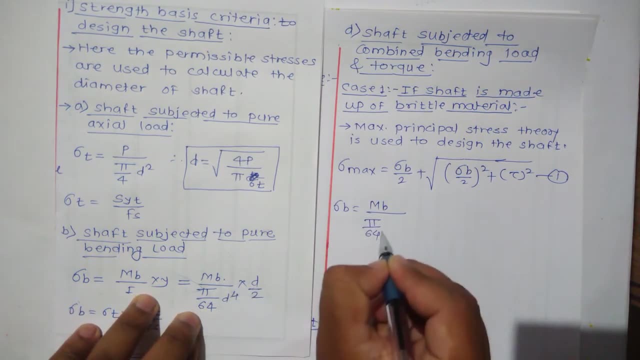 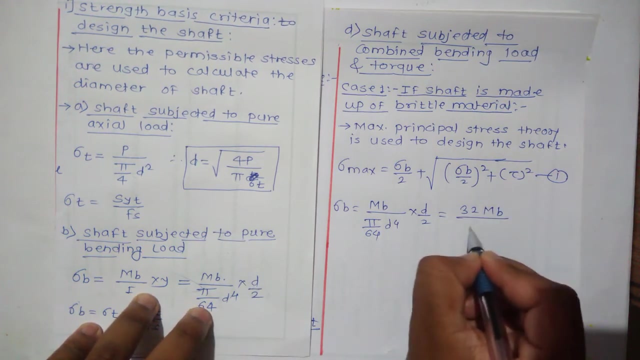 given, as this sigma b is equal to mb upon pi by 64, d raised to 4 into d by 2. if you simplify this because we have already derived the equation of bending stress in the previous steps, so can get the equation of bending stress as 32 mb upon pi d cube, where mb is the bending moment. 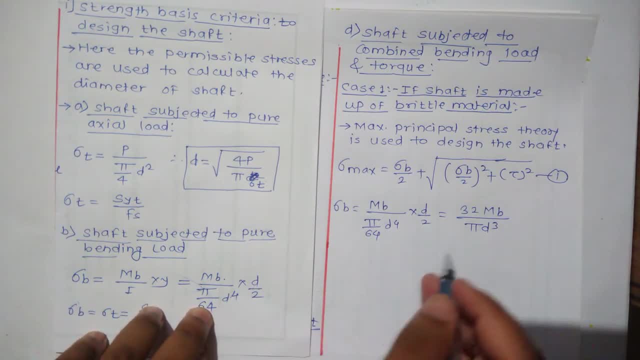 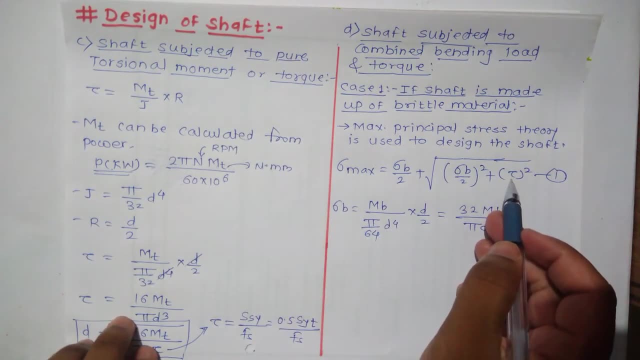 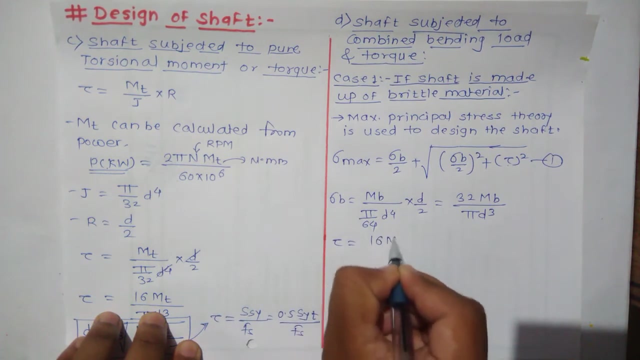 d is the diameter of shaft and sigma b is the bending stress. similarly, we have derived the equation for this torsional shear stress. okay, so torsional shear stress is given by equation. tau is equal to 16 mt upon pi d cube. so if you put the value of bending stress in this equation, 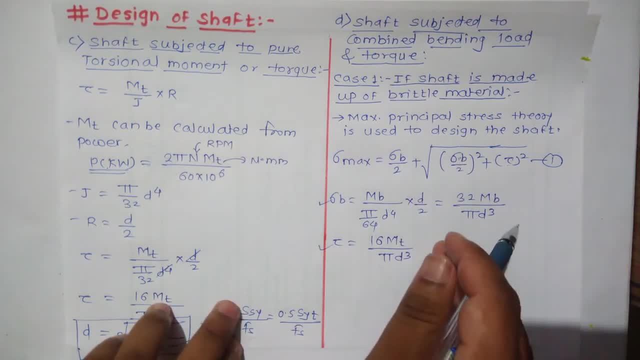 you can get the equation of bending stress as 32 mb upon pi d cube, where mb is the bending moment, d is the bending moment. d is the bending moment, and if we put the value of torsional shear stress in this equation, we can derive the equation to find out the diameter of shaft. so let us put: 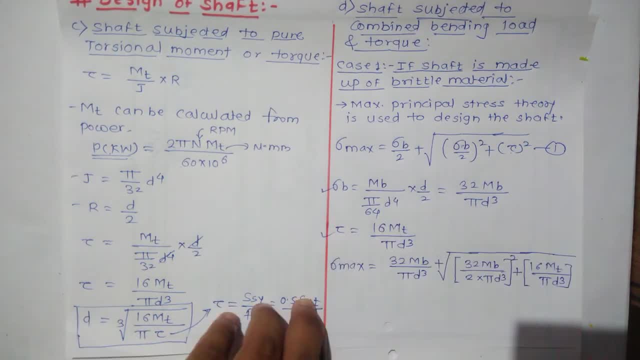 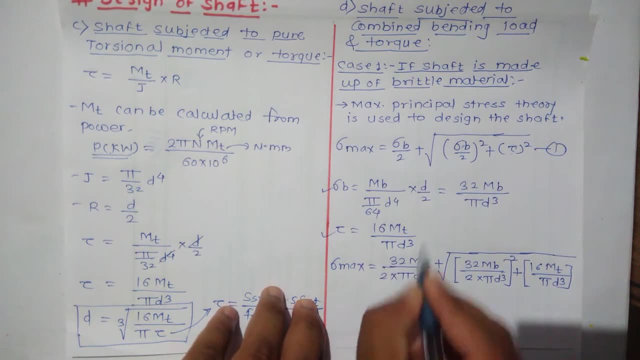 the value of bending stress and torsional shear stress in above equation. so here i have kept the value of sigma b as 32 mb upon pi d cube, so here 2 is we have divided by 2 to this sigma b. so sigma b is 32 mb upon pi d cube upon 2. here also 32 mb upon pi d cube upon 2 bracket square plus tau is 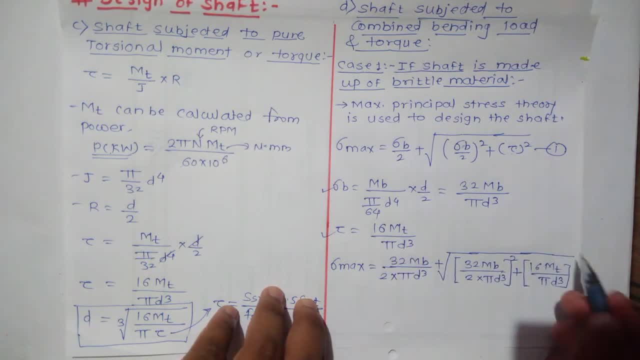 16 mt upon pi d cube. so 16 mt upon pi d cube bracket square. so if you simplify this, you will get here 16, here we get 16 and here already it is 16 mt upon pi d cube. okay, so we can take the 16. 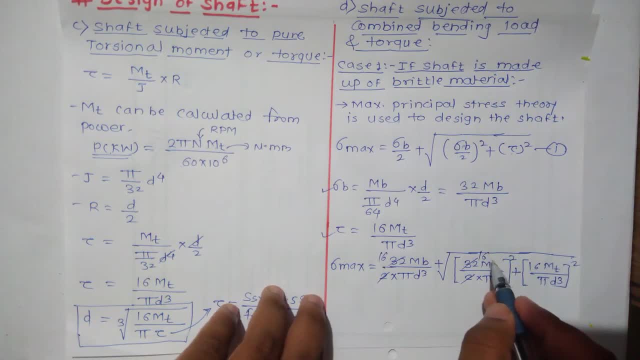 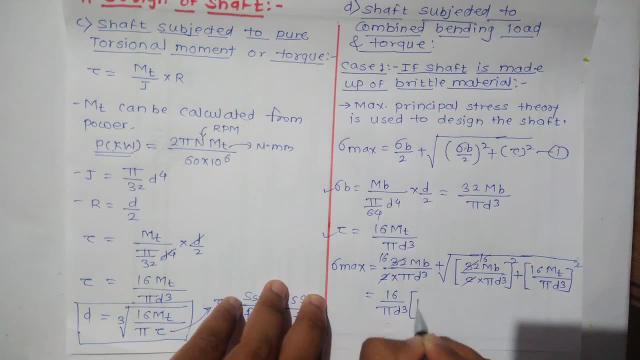 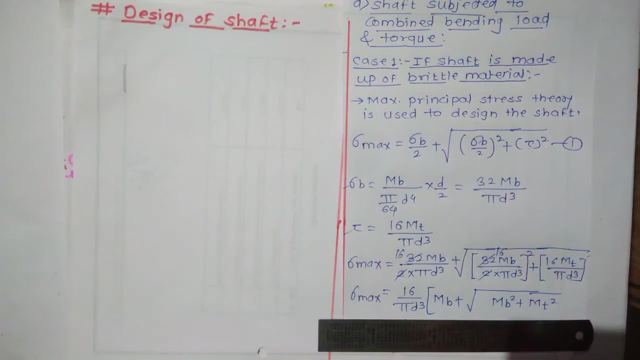 upon pi d cube from this square root common. so we can write here 16 upon pi d cube into bracket mb plus under root: mb square plus mt square. on lhs there is a sigma max. so we have taken the 16, 16 mt upon pi d cube common from this all the terms equation. so this is the important equation. 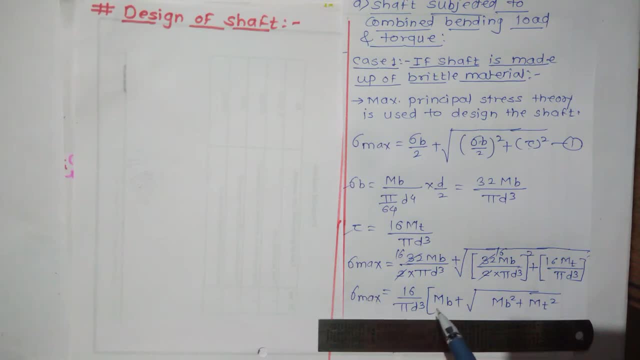 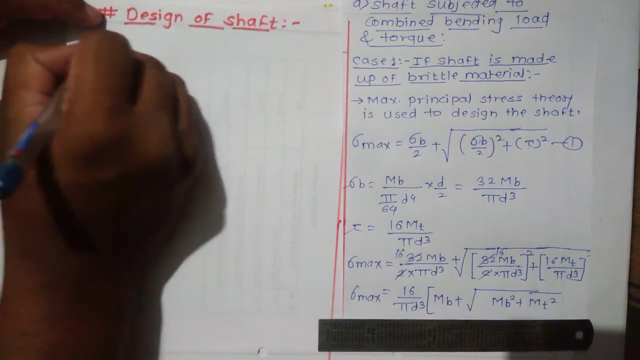 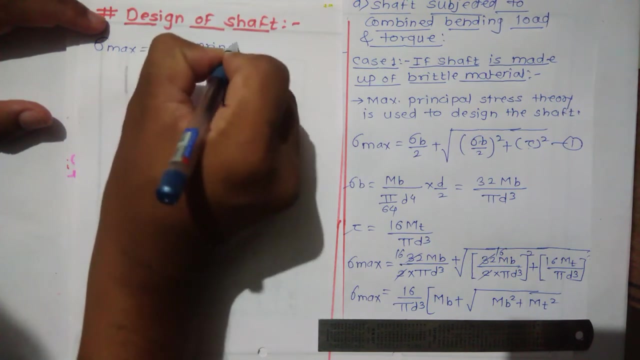 of maximum principle stress, which considers the external bending moment and external torsional moment, that is, torque. now from this equation we can find out the diameter of shaft d by putting the value of this permissible value of maximum principle stress. so this maximum principle stress can be calculated from the equation. so this maximum principle stress can be calculated from the. 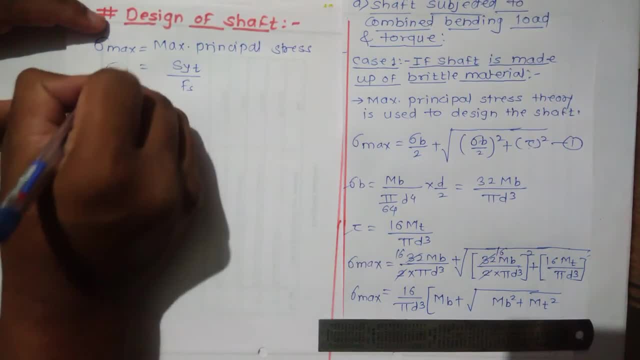 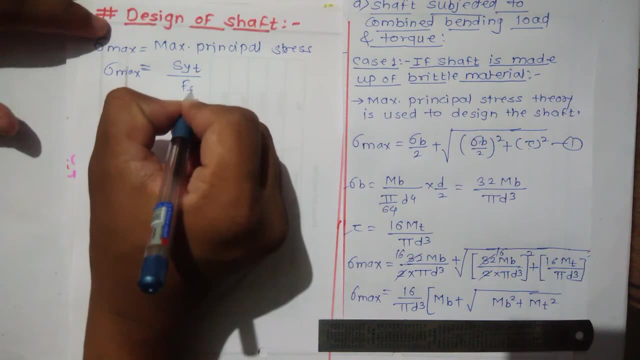 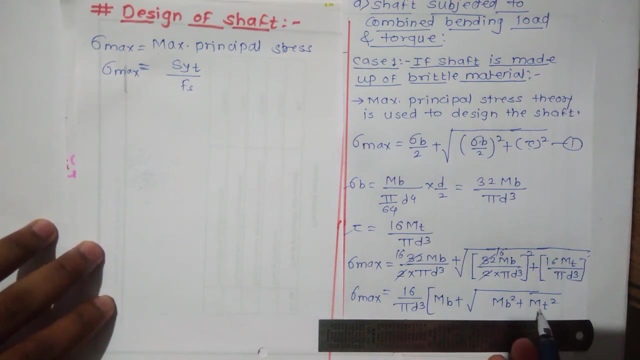 equation syt upon fs, where this syt is yield, strength in tension in newton per mm square, and this fs is the factor of safety. now, next is mb, that is bending moment, and mt is the torsional moment. so by putting the value of this principle, value of maximum principle, stress here, value of bending moment, mb and value, 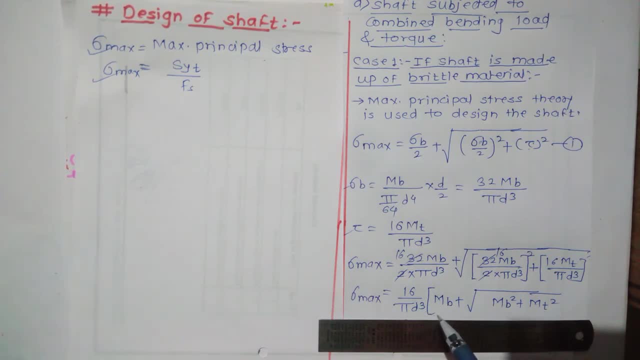 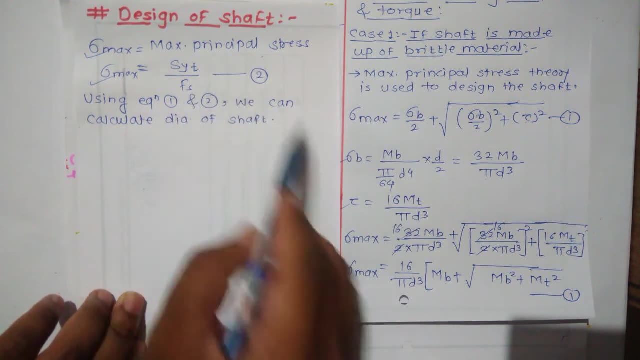 of torsional moment, mt, we can easily calculate the diameter of shaft. so for your understanding, you can give this as equation number one. this is equation number two. so from this equation number one and equation number two you can find out the diameter of sharp, because mb and 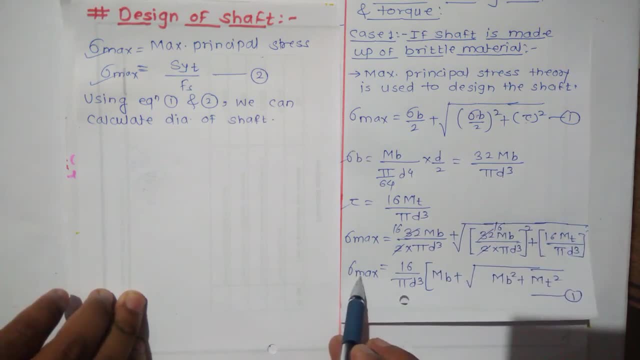 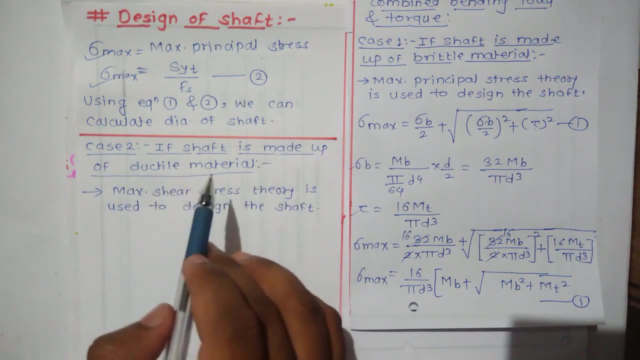 empty, you can easily calculate. so, just you. if you calculate the value of permissible principal stress, maximum principal stress, from this equation number two, you can calculate this diameter of shaft from this equation number one. now let us consider case number two. if the shaft is made up of a ductile material, then we have to use maximum shear stress theory to design the shaft. 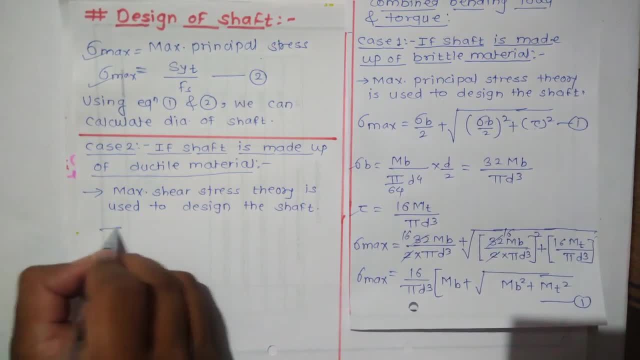 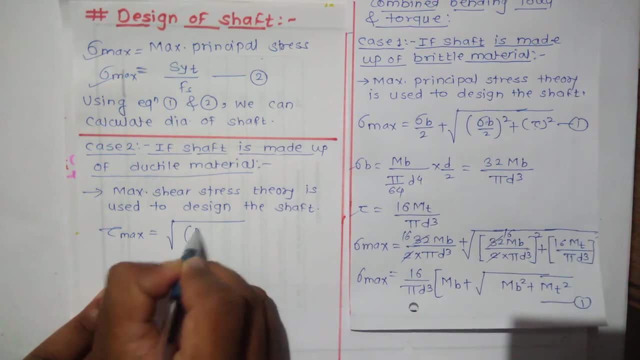 that is to find out the diameter of shaft. now the maximum shear stress down x can be given by equation under root sigma b upon 2 bracket square plus tau square. now already we know that sigma b is 32 mb upon pi d cube and tau is 16 mt upon pi d cube. so let us put the value here and simplify this. 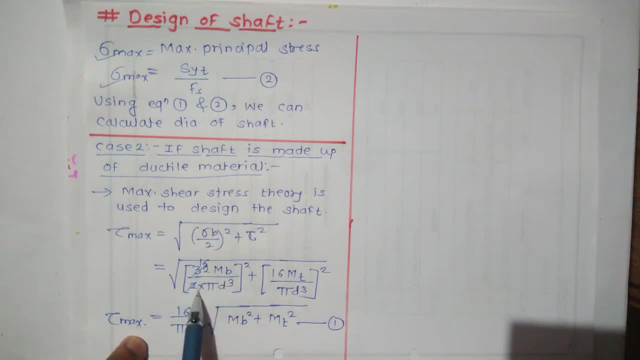 so i have replaced the value of sigma b as 32 mb upon pi d cube upon 2, and tau is 16 mt upon pi d cube. so if you divide this 32 by 2 you will get 16, so you can take common 16. 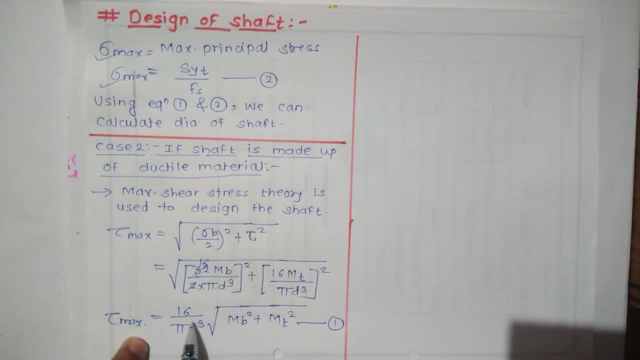 16 upon pi d cube from this square root and its square is there, so you can take this as a 16 upon pi d cube outside the square root and in the bracket or the term remain is mb square plus mt square, where mb is the bending moment and mt is the torsion moment, d is the diameter of. 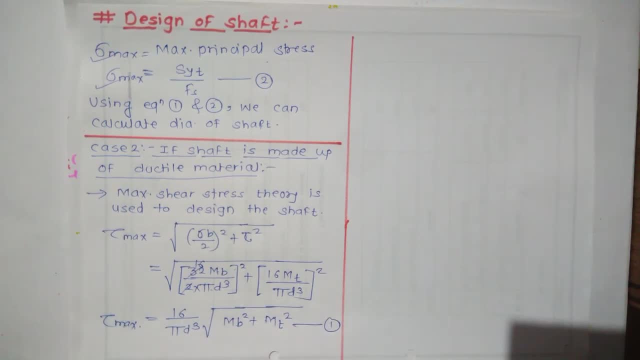 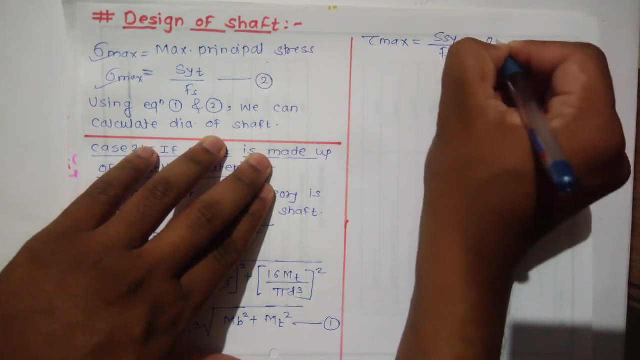 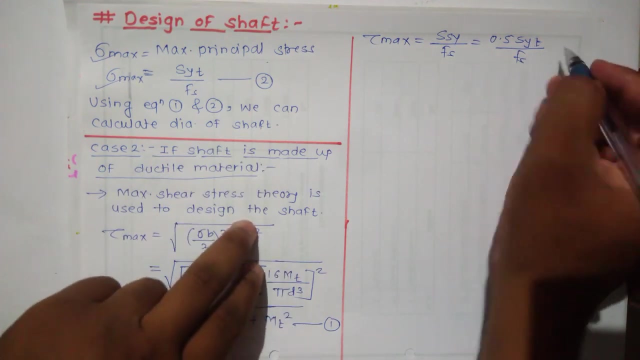 shaft and tau max is the maximum shear stress. now this maximum shear stress, tau max, can be calculated using ssy upon fs, and ssy can be written as 0.5 s y t upon fs, where s? y t is yield strength in tension and fs is factor of safety. so of this is equation number two and this is equation number. 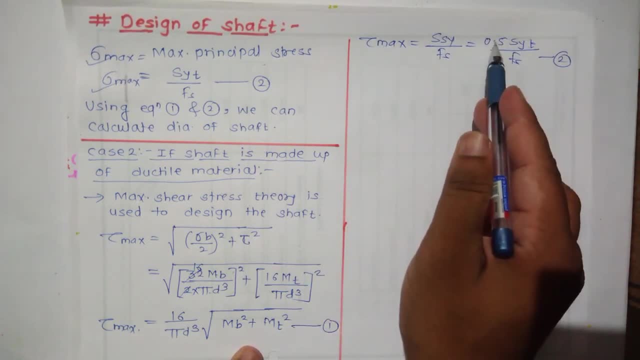 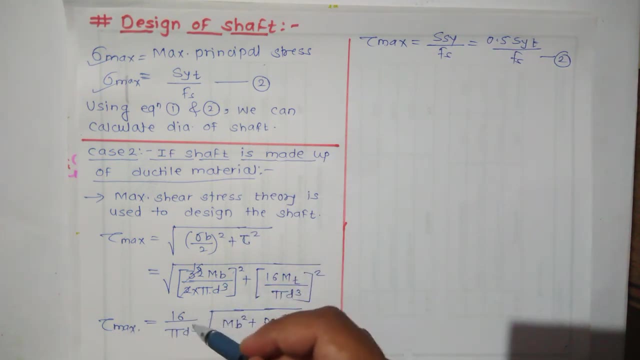 one. so if you put the value of this tau max, which can be calculated from 0.5 s, y, t, upon fs here, if you put the value of mb, if you put the value of mt, you can easily calculate the diameter of shaft. so let us write this. so, with this equation, 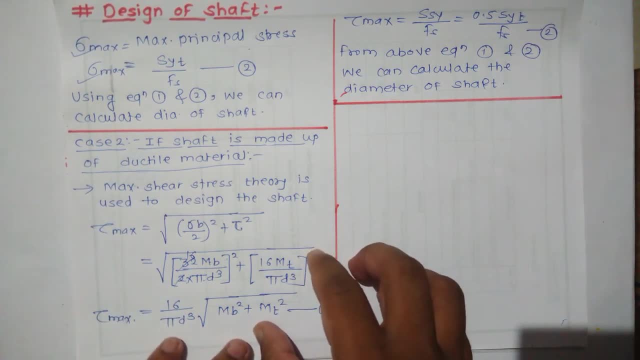 the strength basis criteria to design the shaft is completed. now, after this article, we will discuss about the torsional rigidity criteria to design the shaft.